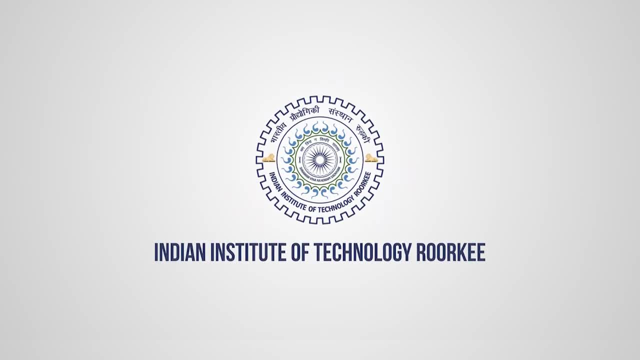 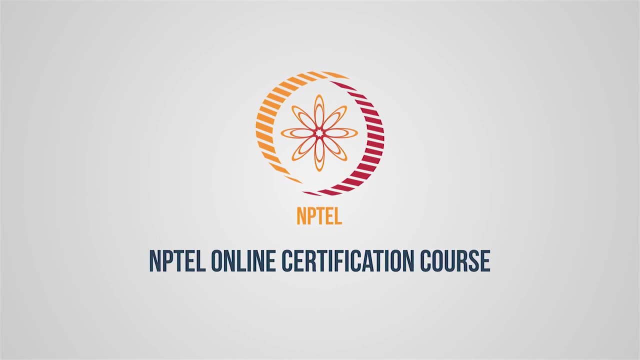 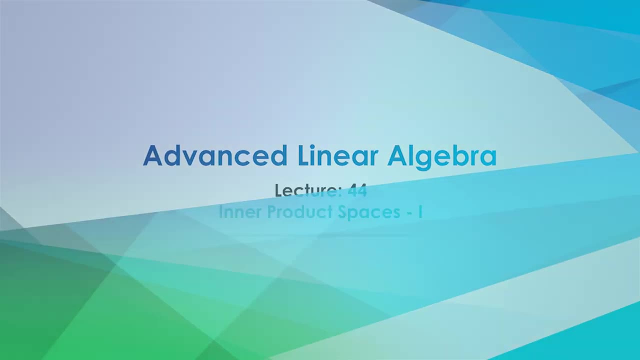 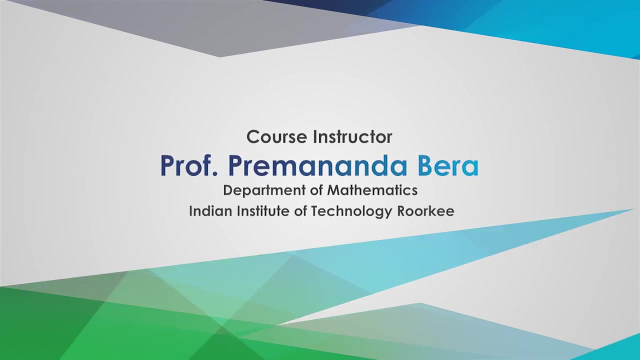 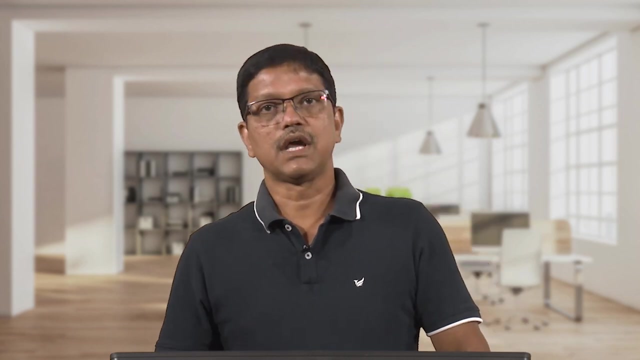 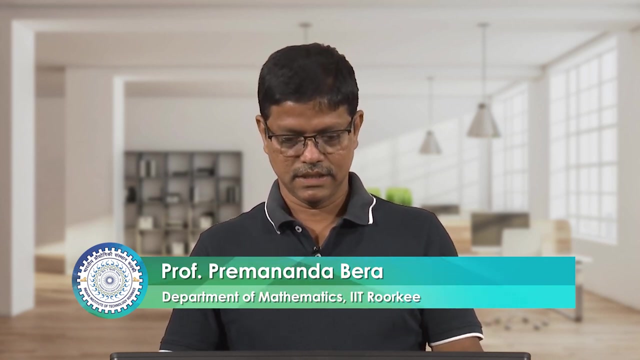 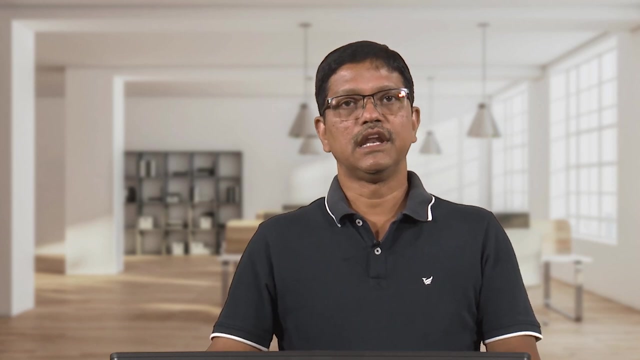 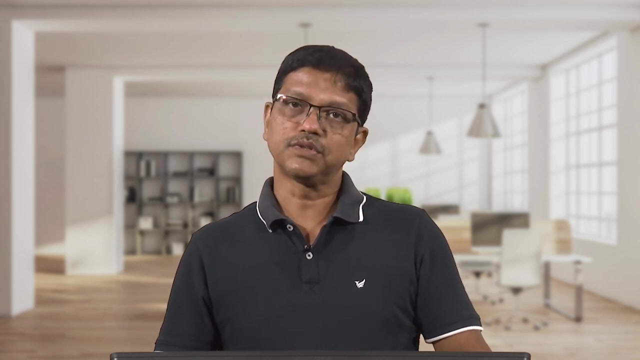 So welcome to lecture series on Advanced Linear Algebra, Friends. we have already learnt the meaning of inner product in a vector space And we have seen how an inner product gives the concept of length of a vector in terms of norm of a vector. We have also seen, within the norm, some important results related to inner product. 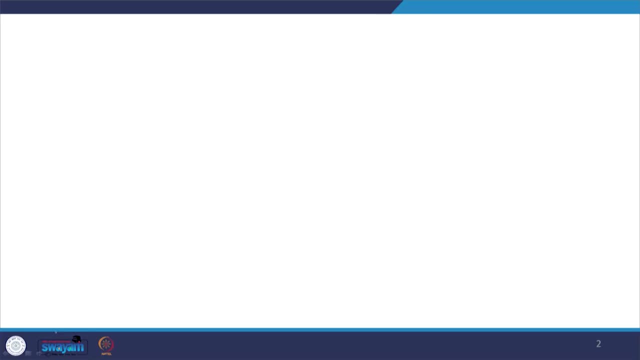 also we have seen like: first is the polarization identity that is inner product of any two vector, alpha beta. If we consider any two vector in a vector space, V, the inner product of alpha beta is equal to. we have seen this is equal to 1 by 4 times sigma n, equal to: 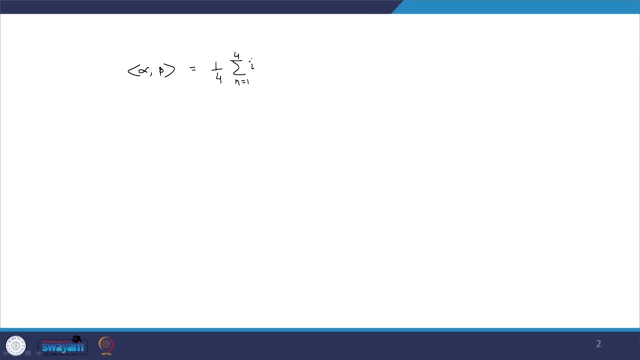 1 to 4.. I to the power n and norm of alpha plus i to the power n beta square. This is called polarization identity, And we have also seen that you know when norm is induced through this inner product. Thank you. product then: norm of alpha plus beta whole, square plus norm of alpha minus beta whole. 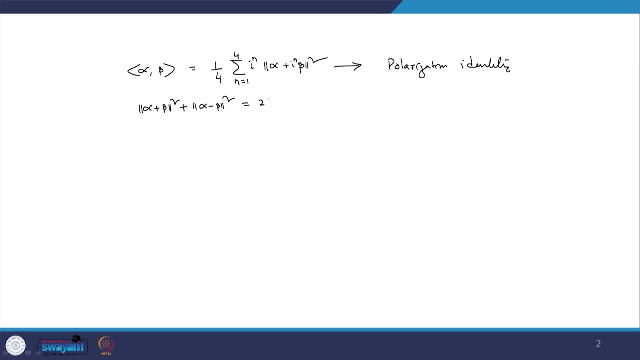 square equal to 2 times of norm of alpha square plus 2 times of beta square. This is called the parallelogram law. See here, norm is induced through the inner product and it is satisfied. parallelogram law and also the inner product of two vector satisfy such type of polarization. 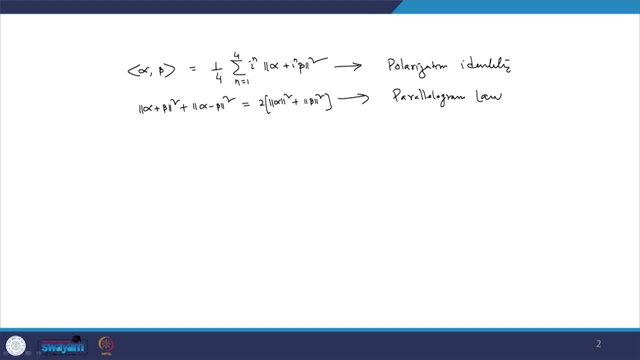 identity. This parallelogram law we will talk about, we will tell you in later on when you are talking or studying in the Mathematical analysis, when we will see that the norm can be introduced by different ways, not through only inner products, Then this parallelogram law will see that only satisfied. 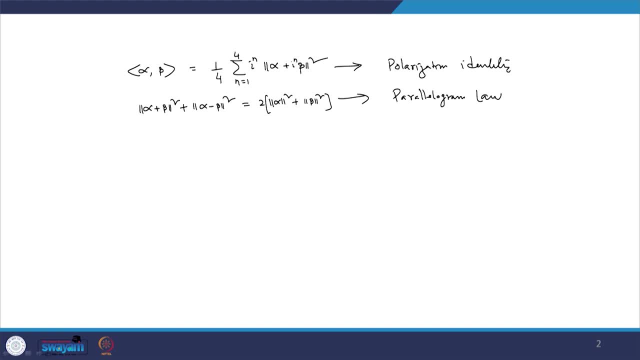 when the norm is induced through inner product only. Another interesting things: we have also seen that when for a finite dimensional vector, space, V for a given order basis, V the inner product, this can be expressed by a, by a, an invertible matrix, Hermitian matrix, which is also positive definite, positive definite, this. 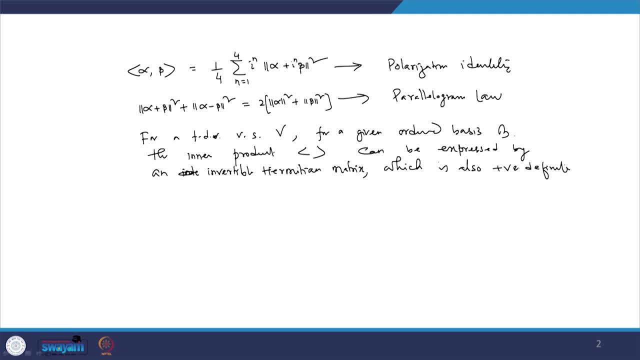 Now we shall utilize this concept of inner product and see the final result. So we will define the combined impact of vector space and inner product. for that, what we will do, I will do. I will first introduce the concept of inner product space. So let me define inner product space, inner product space space. So what is inner product? 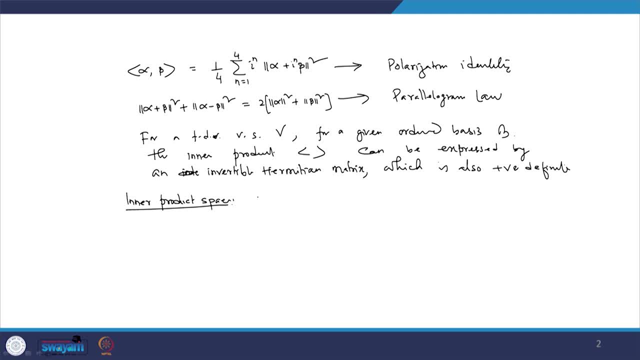 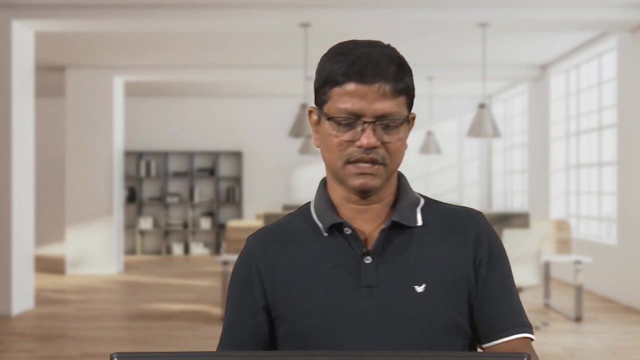 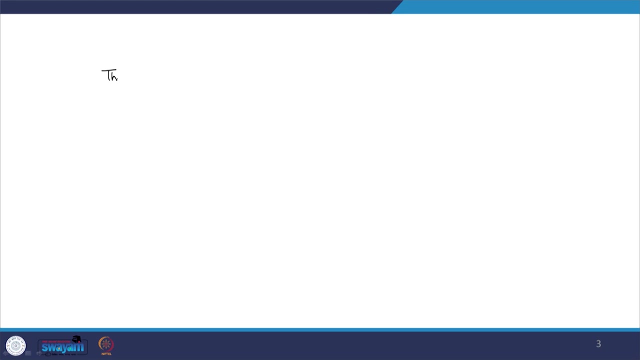 space. So it may be real, it may be complex. place for any alpha. beta belongs to V and C belongs to the corresponding field. field. it may be real number, it may be complex number. Then following properties holds good: 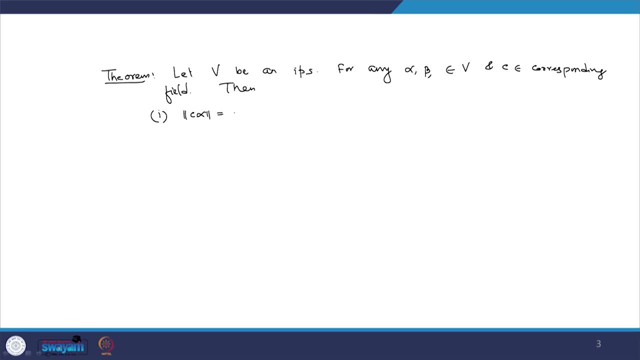 Norm of C. alpha equal to mod of C into norm of alpha. Second, norm of alpha is strictly greater than 0 for alpha not equal to 0.. Third, magnitude of inner product of alpha beta is less than is equal to norm of C. alpha equal to norm of alpha into norm of beta. 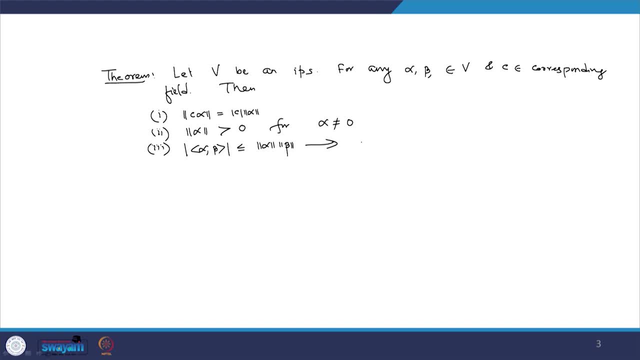 This is called as Cauchy-Schwarz inequality. Cauchy-Schwarz inequality. Fourth one: norm of alpha plus beta is less than or equal to norm of alpha into norm of beta. Okay, Less than is equal to norm of alpha plus norm of beta, please. 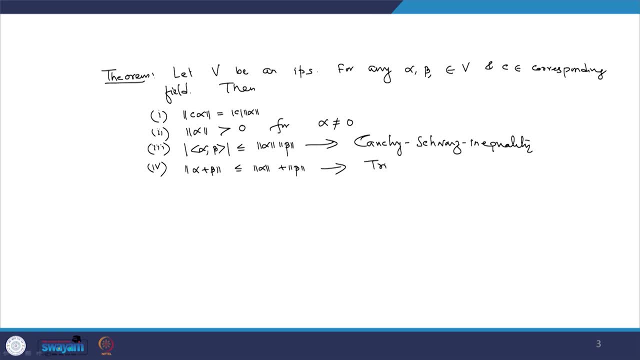 This is is called the triangular inequality. okay, So inner product space V, following four axioms of property holds good, See one. so let me prove one. So let me prove one by one. The first one: we have norm of C alpha square which is equal to inner product of C alpha. 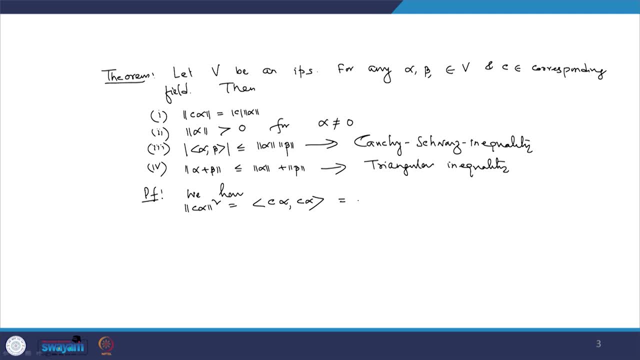 C alpha. This is equal to C into C bar. into alpha alpha. This is equal to mod C whole square into alpha alpha. So this is equal to norm of C alpha square is equal to norm of C alpha square into C alpha, into norm of alpha square. 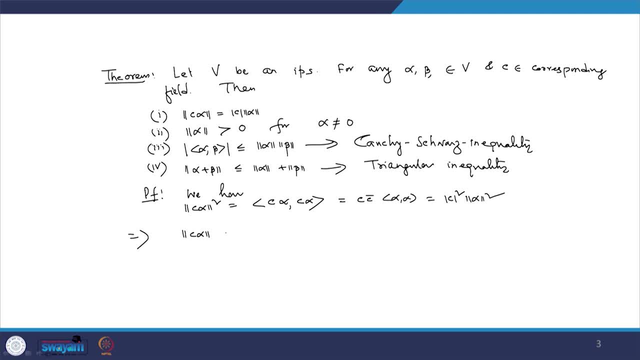 So this implies norm of C. alpha, which is a positive quantity, should be mod of C into mod of alpha. And second one is satisfying since inner product of alpha alpha is strictly greater than 0, for alpha not equal to 0 implies norm of alpha square is strictly greater than 0.. 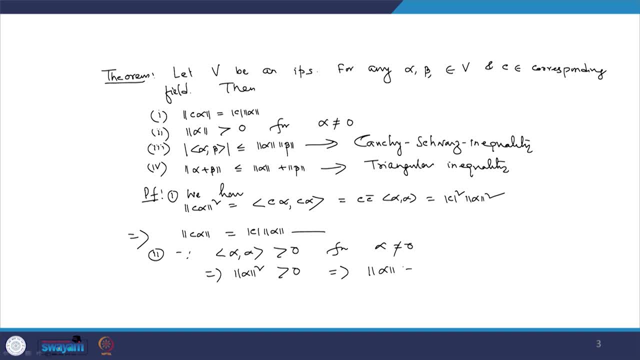 So this implies norm of alpha is strictly greater than 0 for alpha not equal to 0.. Third one, that is Cauchy Schwarz inequality. for this we have to show magnitude of inner product of alpha beta. It is less than or equal to norm of alpha into norm of beta. 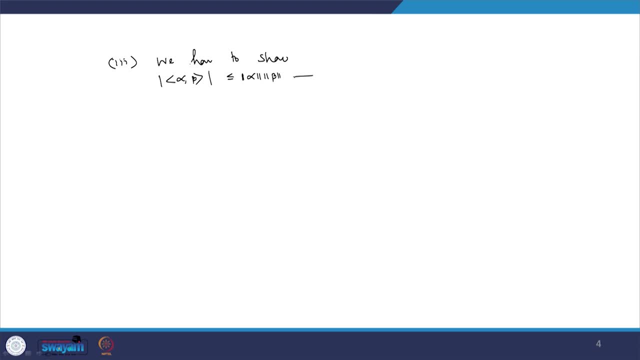 See, if alpha equal to 0 or beta equal to 0, then this inequality definitely satisfied. So let alpha not equal to 0 and beta not equal to 0. So for this case we have. Let me consider gamma. Gamma is another vector- is equal to beta minus inner product of beta and alpha divided by. 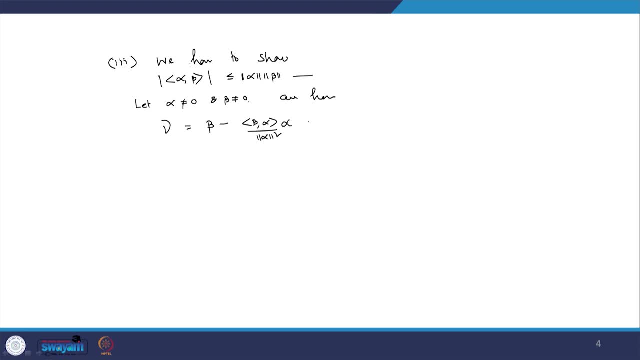 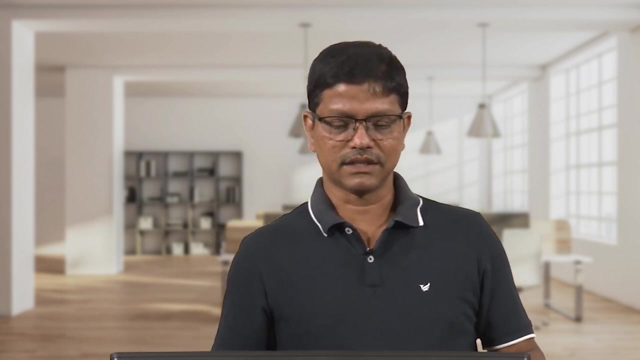 alpha square into alpha. You may raise the question how to think that I have to consider gamma equal to like this. I will answer this question in my next- I mean coming soon- basically, when I am talking about this- another terminology that is called orthogonality of the vector piece. 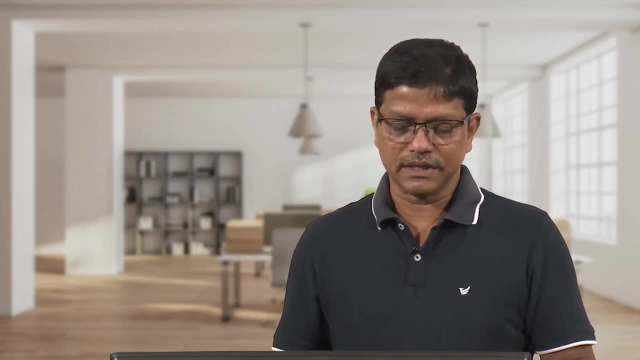 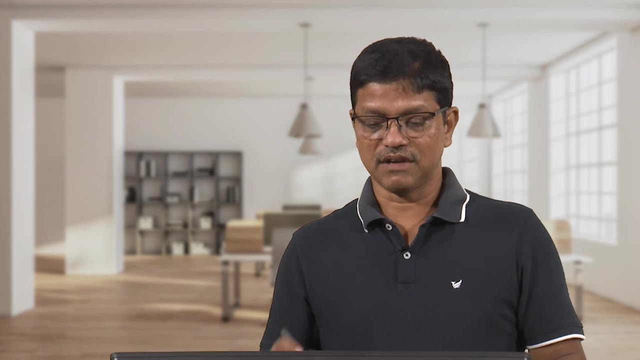 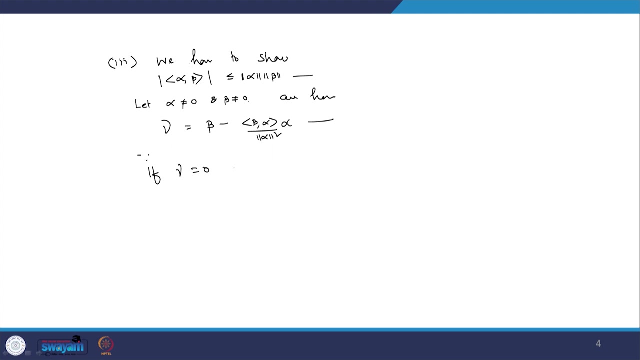 Thank you. So now I have taken, gamma is another vector, so it is basically beta minus inner product of beta. alpha by norm of alpha square into alpha. So we have, if gamma equal to 0. this implies that beta can be written as a scalar multiple. 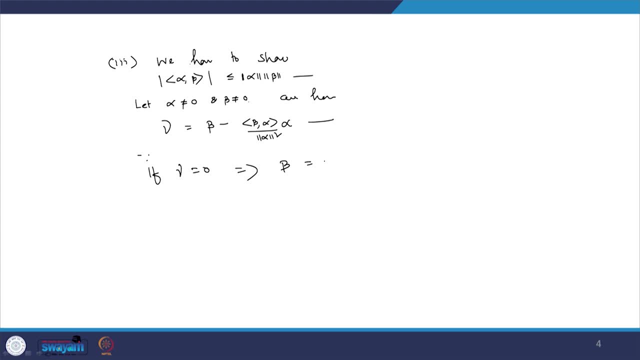 of alpha. This implies beta equal to inner product of beta alpha by norm of alpha square. This is a scalar quantity, so beta is basically a scalar product of the alpha piece. Now let me consider beta not equal to Let beta not equal to beta alpha. by alpha I mean beta not equal to simply a scalar multiple. 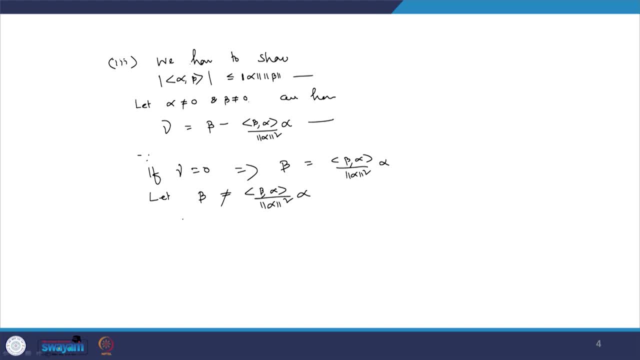 of alpha. So In that case, so gamma not equal to 0. in that case, So gamma not equal to 0 means ok, We have inner product of gamma and alpha. let me check that one inner product of alpha, gamma and alpha equal to inner product of beta minus beta. alpha square into alpha. square into alpha. 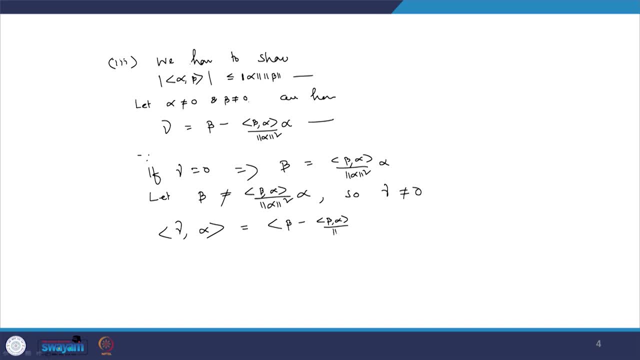 square. So let me write here that I have to make in a relationship between alpha and beta and alpha. then I have to make sure that an рав vai alpha- here, sir, it is super clear- alpha can be write, or, if you want to write it in any other way, 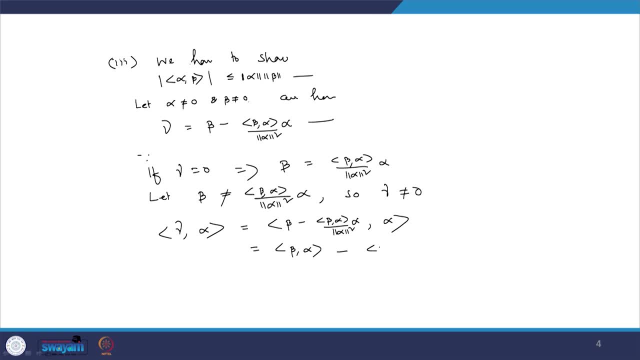 So it is equal toちょっと ask multiple times better answer, and then it is always a. the Future got what I mean. So this can also be written as dash greater than- for distance and-. this can also be written as dash greater than- the. therefore, this is my default mistake. 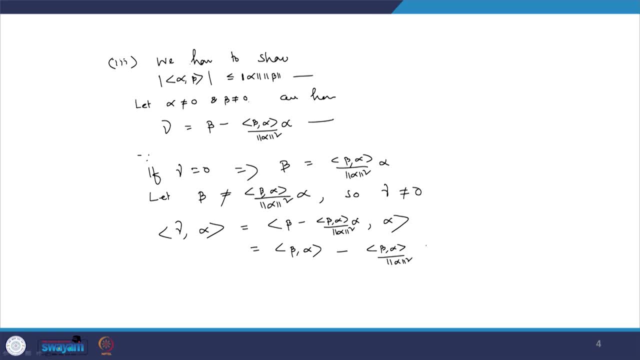 if you take, for instance, alpha is equal to. that is also true is to say alpha is equal to daughter of beta alpha, right altele six plus beta, alpha and alpha. So this is called to inner product of beta alpha minus inner product of beta alpha by. 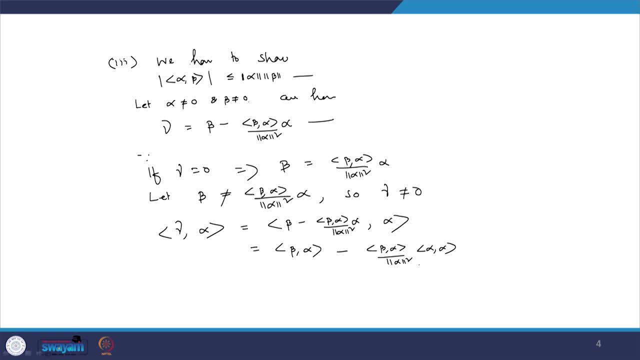 alpha square into a broader alpha. So I have used basically the property of the definition of the inner product. from that I that inner product of gamma alpha, like this. So this is equal to, you see, inner product of beta alpha minus inner product of beta alpha only. So this is equal to 0.. So this: 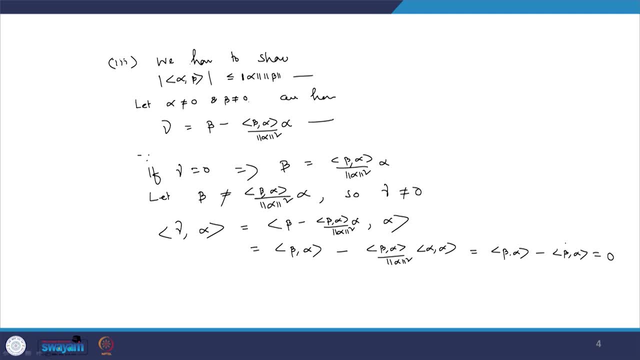 implies that we have considering vector gamma, such that inner product of gamma and alpha equal to 0. We have 0 is strictly less than gamma and gamma inner product of gamma gamma, because if I have considered gamma not equal to 0. So gamma not equal to 0. So this means 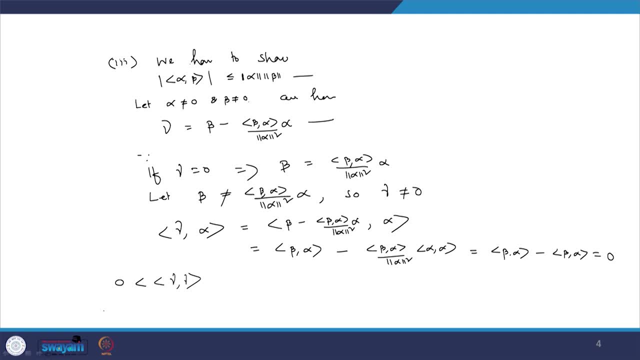 that inner product of gamma gamma is strictly greater than 0. I mean this will be equal to inner product of your gamma and I can write on beta minus inner product of beta alpha by norm of alpha square into alpha. So 0 less than inner product of gamma and gamma is equal to inner product of gamma, beta and 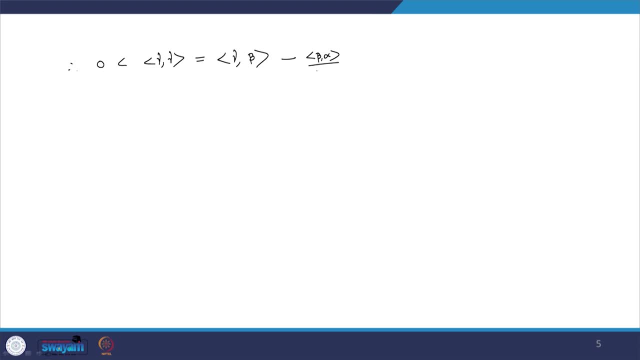 minus inner product of beta, alpha by norm of alpha square and gamma and alpha please. So we have inner product of gamma, gamma that is equal to this square, but this is equal to 0 already. we have seen it. So this is equal to 0.. So this implies that 0 is strictly. 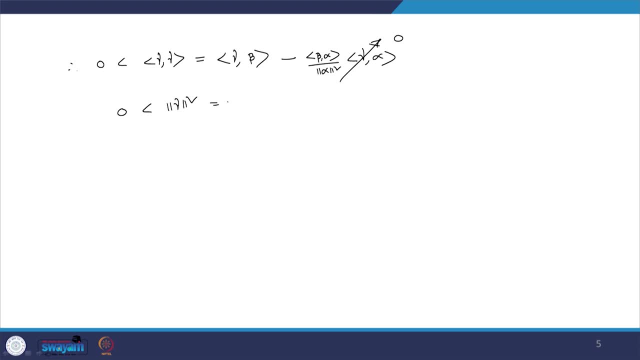 less than norm of gamma square, which is equal to inner product of gamma and beta please. And that is equal to, again, according to the definition of the gamma, this is equal to beta minus inner product of beta alpha by alpha square and alpha and then beta please. So 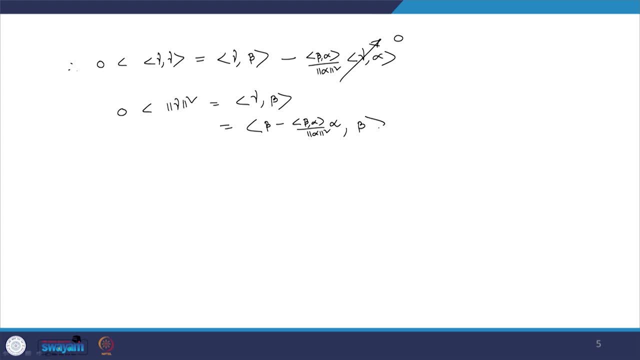 this is equal to 0.. So this is equal to 0.. So this implies that 0 is strictly less than norm of gamma times beta after getting out of this square. This is also by norm alphapeta beta, but nya take this as 1 betaなた. 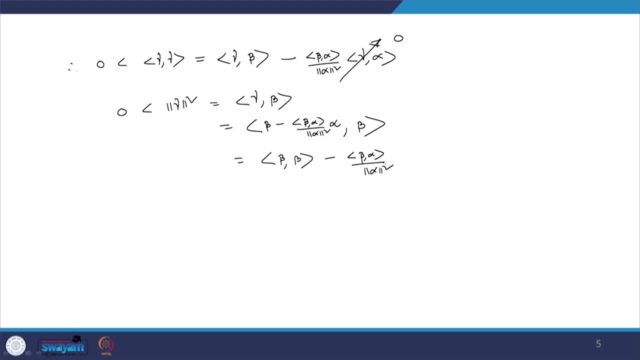 This is my assumption by norm alphapeta plus of 0. So I take the derivative part of the problem as 0 Planar Poisson or 1 Planar Poisson. This is also equal to 0. this is equal to 0. and this is basically a cooperative coefficient of all theosi of a 0 Planar Po knitting. So by norm of beta, which is blanket. So I refresh the Data and then beta please. So this is equal toWill Savor the Leimont equation at alpha. So this is equivaler toinner product of beta, beta and minus the Shore. 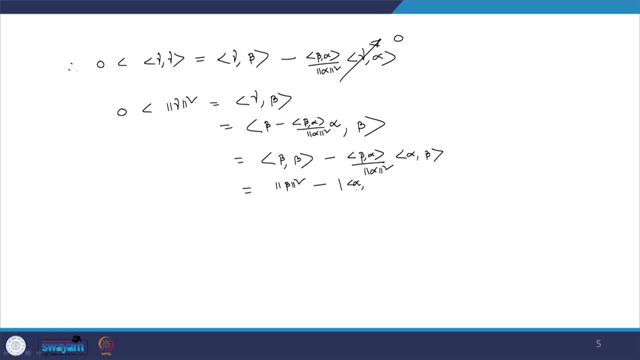 absolute value of inner product of alpha and beta, this whole square place and divided by norm of alpha square. So this implies that 0 less than norm of beta square into norm of alpha square minus inner product of alpha beta whole square. So here I have taken 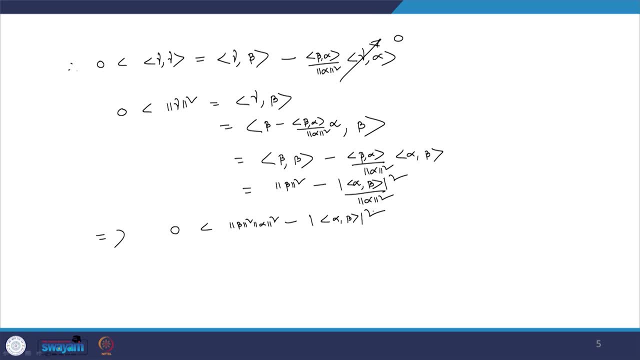 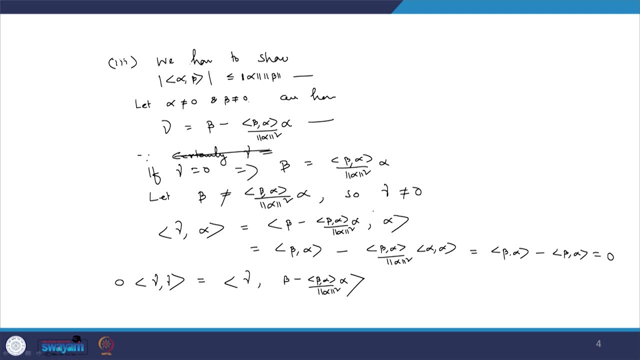 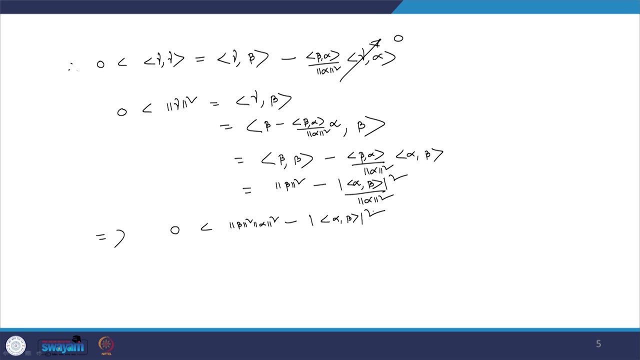 this strictly less than 0, strictly less than this. quantity based on gamma not equal to 0, please. gamma not equal to 0 and gamma not beta not equal to again. linear scalar, multiple of alpha, please. ok. So if you do not calculate, 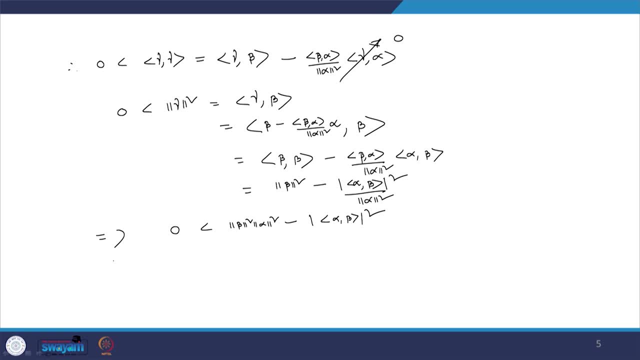 Consider that one, then it will be less than equal to also please. So this implies that I will have mod of inner product of alpha beta. whole square is less than norm of beta square and norm of alpha square, please. This implies mod of inner product of alpha beta. 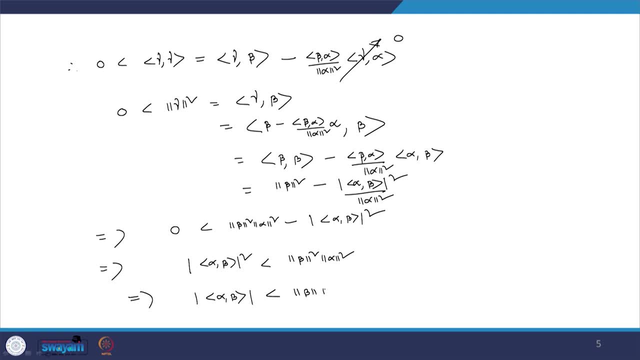 will be less than norm of beta square. This implies ici alpha by beta, by norm of alpha, by sm boss square multiplied by alpha square. it comes to som Network Anyhow, so equivalinity will come into the picture if we consider that beta equal to. 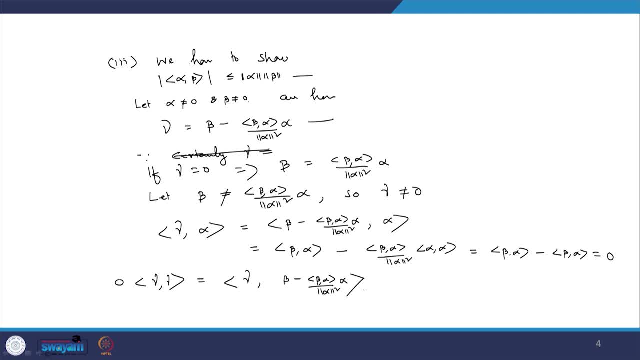 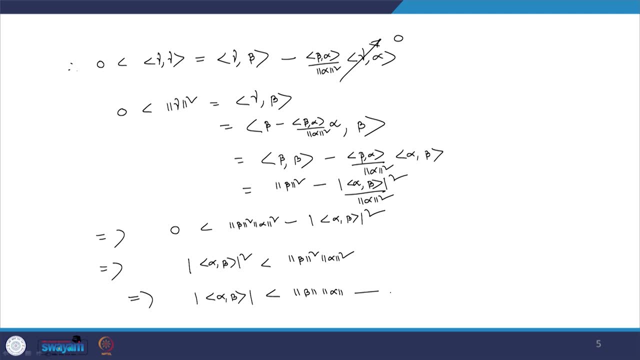 inner product of beta alpha. by alpha square into alpha plus, I mean scalar multiple of alpha. so in that case equal will come to the picture, please. ok, The next result was that triangular inequality cuál. We have to show that norm of alpha plus beta is less than or equal to norm of alpha plus. 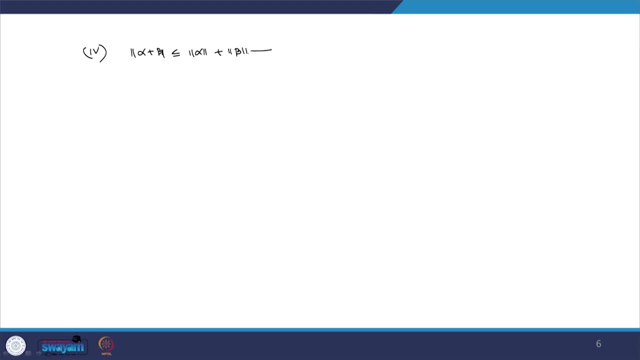 norm of beta. So for this we have- we have see norm of alpha plus beta whole square. that is equal to norm of alpha square plus norm of beta square- already we have proved it- plus 2 times real part of beta. So this implies norm of alpha plus beta whole square will be less than or equal to norm. 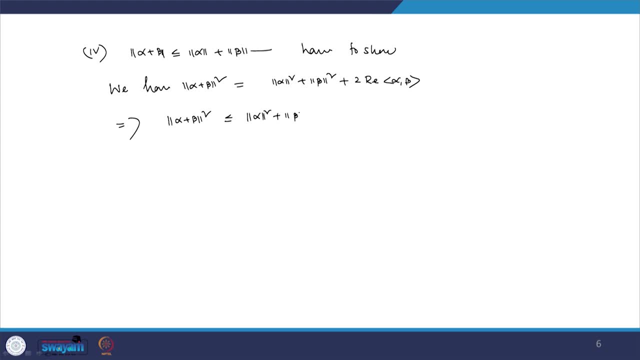 of alpha square plus norm of beta square plus 2 times of real part, I will say absolute value of the inner product of alpha beta. So I can say real will be vanish because we have taken the absolute one. So I will say that 2 times of inner product of alpha beta, please. absolute value of the. 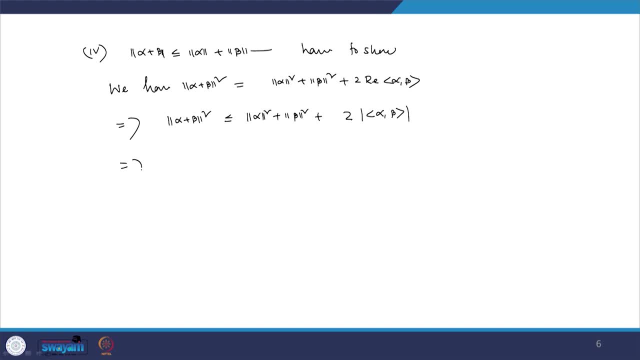 inner product of alpha beta, please. So this implies that this is less than equal to norm of alpha square plus norm of beta square plus norm of beta square. So this implies, if it is 2 times 2 by conscious Schwarz's inequality, that is from 3 already. 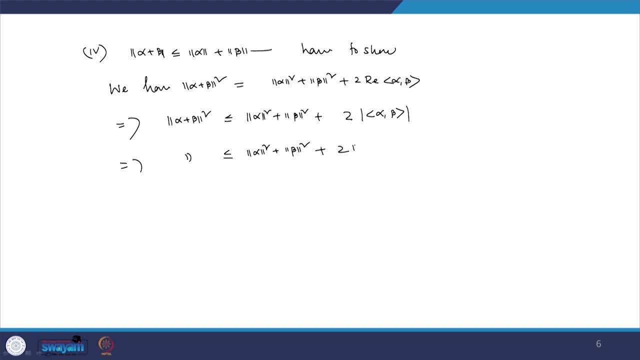 approved we will have. this is less than equal to norm of alpha into norm of beta. So this is equal to norm of alpha plus norm of beta, a whole square. So this implies norm of alpha plus beta is less than or equal to norm of alpha plus norm. 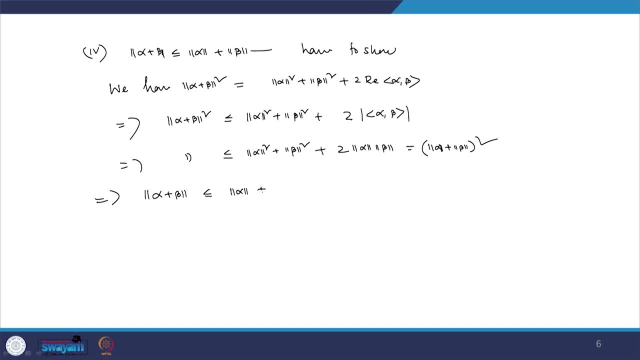 equal to norm of alpha plus norm of beta. This is triangular inequality place. So you will see the application of 3 and 4 is rigorous. In many places we use Cauchy-Schwarz inequality. we also use the concept of triangular inequality place. 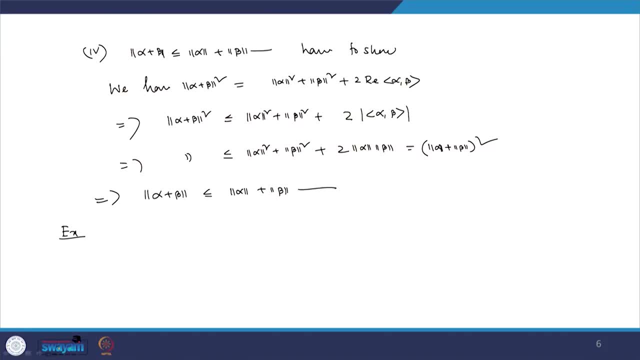 Now let me consider some example. place Let V is equal to. let me consider V may be, say F n, space of n tuples. Here this field is real number or complex number. place Let inner product is standard inner product, Standard inner product on F n. So let alpha which is equal to x 1, x 2, x n and beta equal to y 1,, y, 2, y. 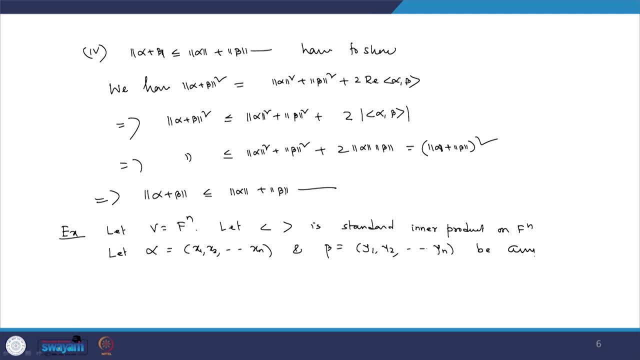 n be any two elements of x 1, x 2, x n and beta equal to x 1, x 2, x n. So let alpha V equal to F n, Then inner product of alpha beta, then we have inner product of alpha. 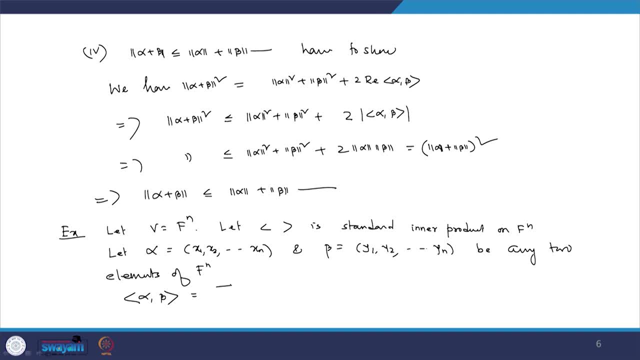 beta equal to sigma x, j, y, j, bar. j equal to 1 to n place. So this implies: mod of inner product of alpha beta is equal to x, j, y, j, bar. j equal to 1 to n place. So sigma j equal to 1 to n. x, j, y, j bar this quantity place. So, according to the 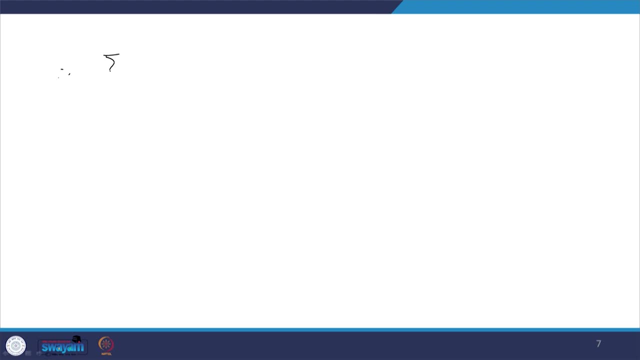 Cauchy-Schwarz inequality summation: j equal to 1 to n, x, j, y, j, bar this quantity, So the product of alpha will be less than equal to inner product of alpha and inner product of beta. Inner product of alpha is equal to j. equal to 1 to n, x, j into x, j, bar that is. 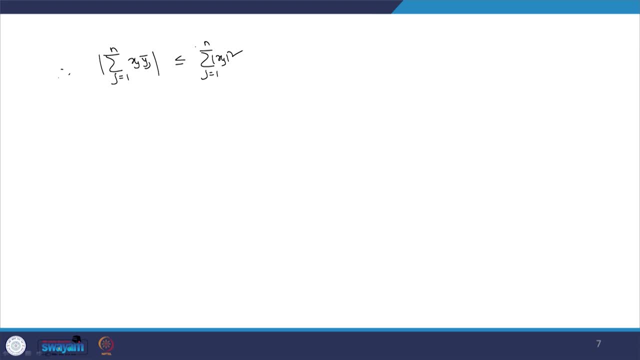 x, j square, that is, I can say mod of x square. This whole power 1 by 2, inner product of alpha, alpha square root, positive square root to that one, into again mod of yj square, j equal to 1 to n. this whole power 1 by 2 place. 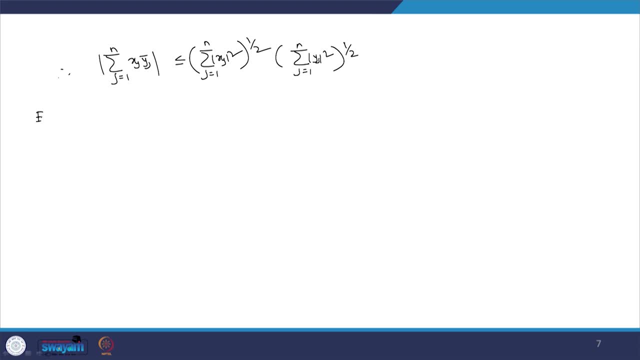 Now this is over. our fn now over. let me consider another examples. that is, a space, of say, continuous function. say let V be the space of real or complex valued continuous function on the close interval 0, 1.. And let the inner product in V be defined by: for any f and g belongs to V inner product. 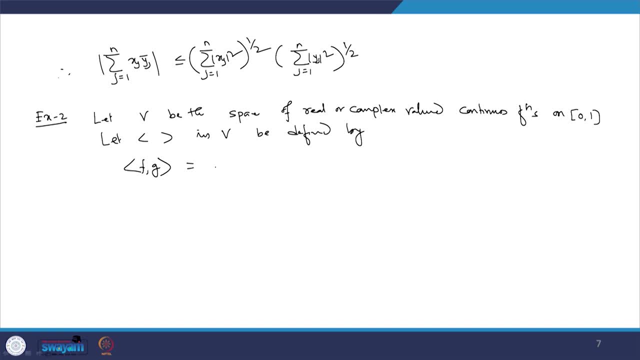 of f and g. let me write down: this is equal to your 0 to 1 f of x and g, of x bar dx. So this is the inner product of f and g. any two elements of this one place Now, according to this, Cauchy Schwarz inequality. so using Cauchy Schwarz, inequality, C, S, inequality. 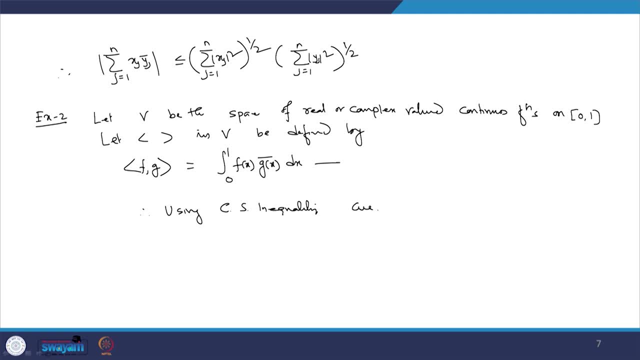 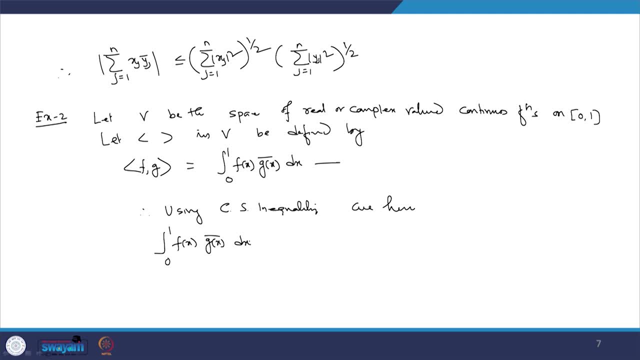 gx dx. this is less than equal to. I will say that absolute value is less than is equal to inner product of f and f. So that is equal to 0 to 1 mod of f of x, whole square dx, whole power 1 by 2. and again, integration of 0 to 1 mod of gx, whole square dx power 1 by 2.. 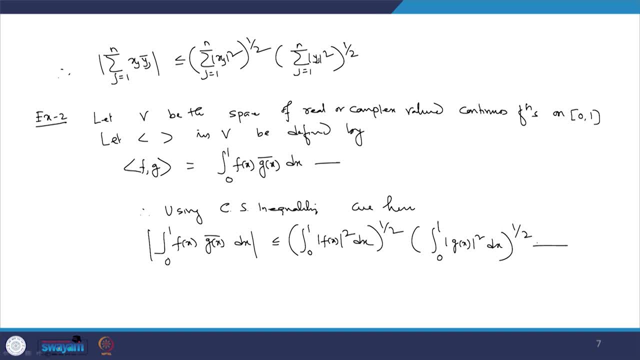 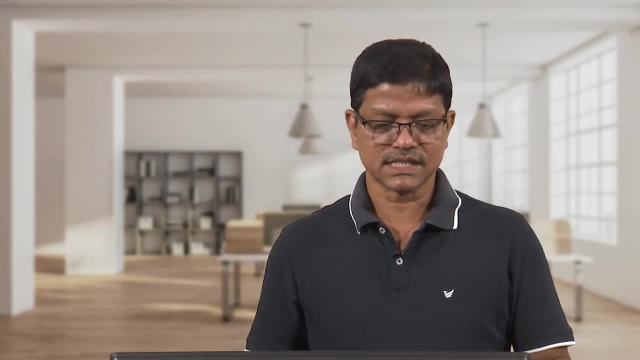 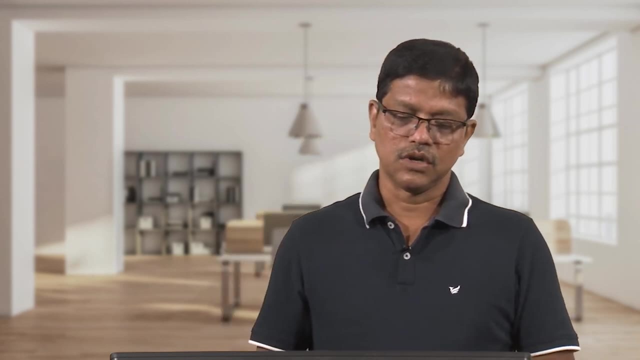 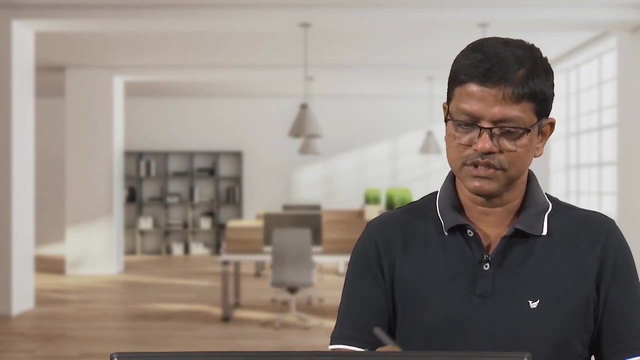 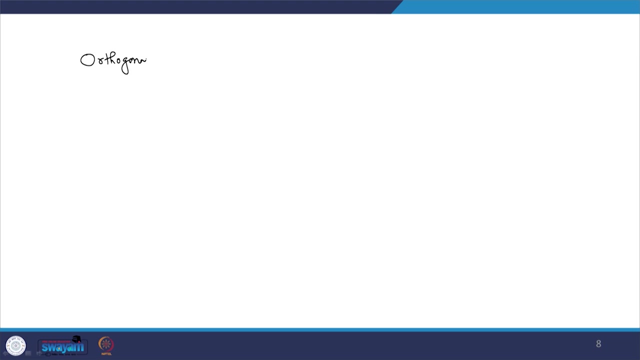 So we can. we will discuss more problems in my next classes, So I hope the concept of this inner product space And some properties in inner product space is clear. Now let me introduce one more terminology, interesting terminology called orthogonal vectors. please, orthogonal vectors, Let V b. 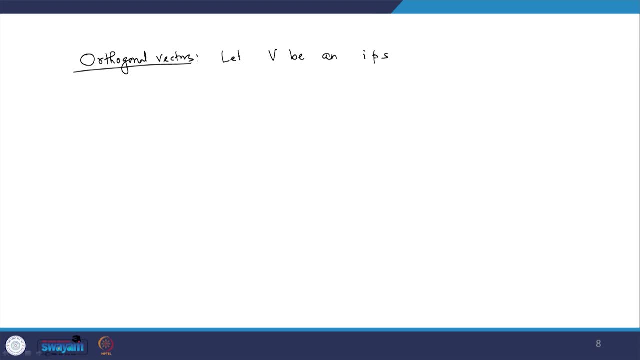 n- inner product space. Let alpha and beta be any two vectors. in V, Beta is said to be orthogonal to alpha provided inner product of alpha beta equal to 0. So beta will be orthogonal to alpha provided inner product of alpha beta equal to 0.. If inner product of alpha beta equal to 0, then 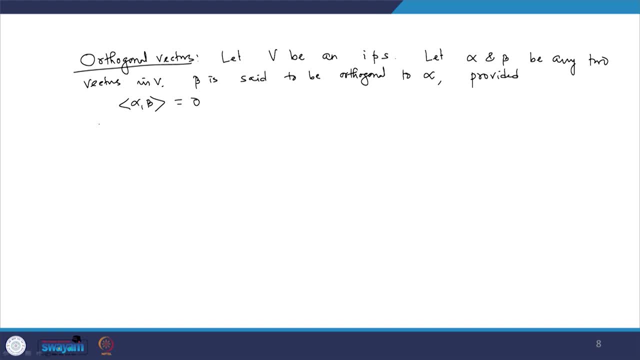 inner product of beta alpha equal to also 0. So this implies alpha is also orthogonal to beta. please. orthogonal to beta, please. For example, let me consider: let V is equal to my R 2 space and let me consider the standard inner product on E as a. this is a standard. 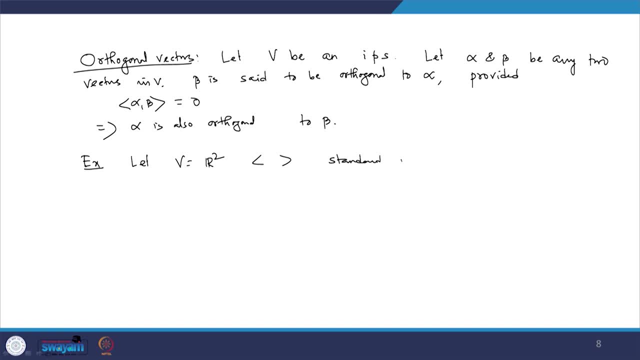 inner product: standard inner product. ok, So let alpha equal to x comma y. So we want to know an element beta in V which will be orthogonal to alpha. So immediately I can see that then beta which is equal to minus. 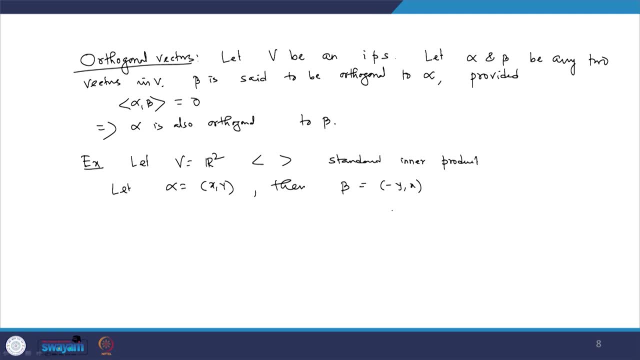 y, x or y minus x will be orthogonal to alpha. So inner product of alpha beta is equal to x. into minus y plus y into x is equal to 0.. If I consider over the same space, let me change the inner product. Let inner product. 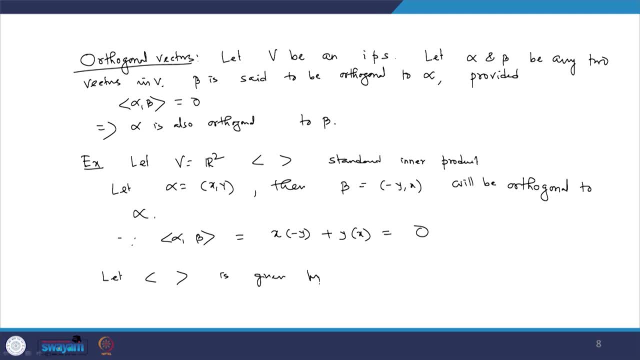 is given by like this, that let me consider say So, alpha equal to x 1 x 2 and beta is equal to say y 1 y 2, and let me define inner product as inner product of alpha: beta equal to x 1 y 1 minus x 2 y 1 minus x 1 y 2 plus 4 x. 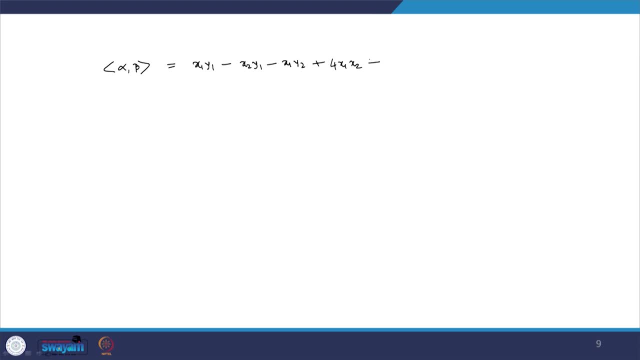 1 x 2.. So already you have seen this introduce and dans product over the R 2.. Now if alpha equal to- let me consider x, y and beta is equal to say minus y. x is orthogonal to alpha, then x 1.. Let us leave it like this. So this is the結föriesta. So in this particular theorem we have already seen this introduce an inner product over the r 2.. So already we have seen this introduce an inner product over the r 2.. 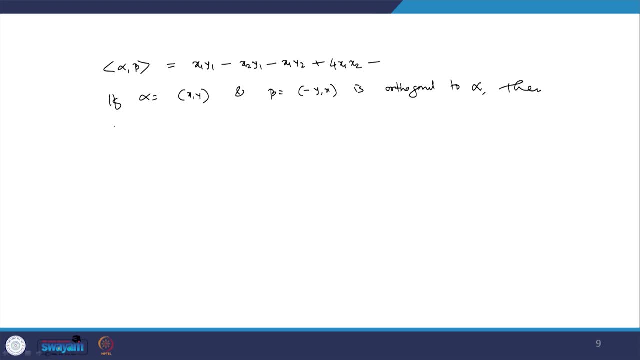 Now, if alpha equal to- let me consider x, y and beta is equal to say, minus y, x is orthogonal to alpha, then We will definitely have inner product of alpha and beta will be equal to 0. But in this case, what I am getting here? if I consider that, as in the case of the previous, 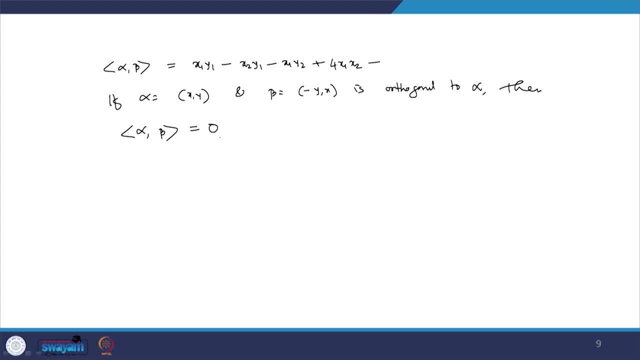 one what the standard inner product space that are for alpha equal to x, y, beta equal to minus y, x is orthogonal. So here, beta equal to minus y, x will be orthogonal, provided let me see what are the conditions. So this is equal to 0, means x into minus y minus x2, that is, y into y1 means minus y. 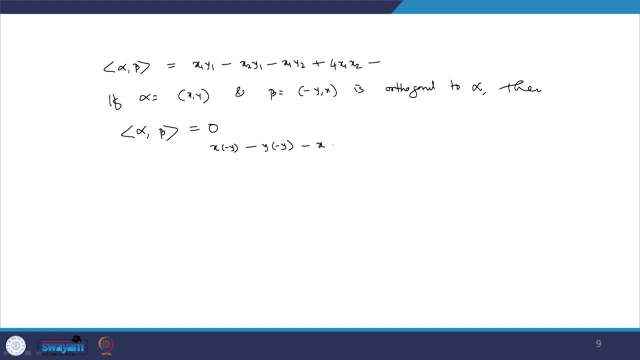 Then minus x1, that is x into, and y2 means x. Okay, Okay, Then plus 4, x1, that is x, and x2 means again x. this is 4: x2, y2, x2, y2.. So this means that y2 equal to x. 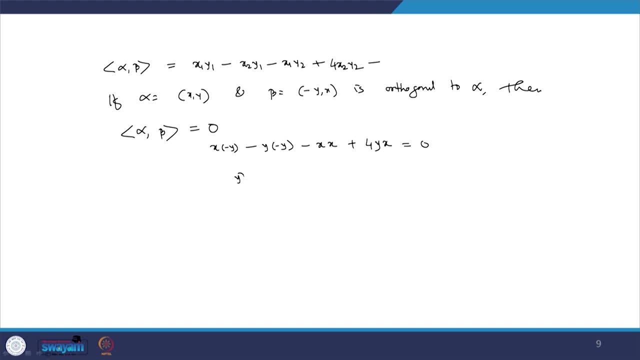 So this is equal to 0.. So this means that I am getting y square minus x square plus 3 yx, equal to 0.. So from this, So from this, we can have a relation between y and x, for which that alpha and beta will. 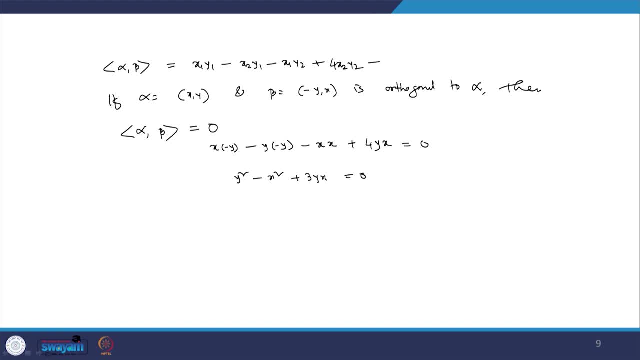 be alpha will be orthogonal to beta, or beta will be orthogonal to alpha place. So one can have immediately here: y will be equal to minus 3x plus minus root over square 9 x square and 9 x square minus 4ac. 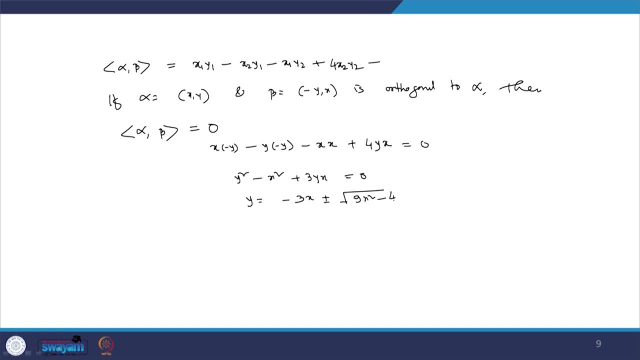 Okay, Okay, Okay. So that is 4 into x square, right, that is plus by 2.. Okay, some sort of this relation will get it place, So something like minus 3x plus minus root over 13x by 2.. 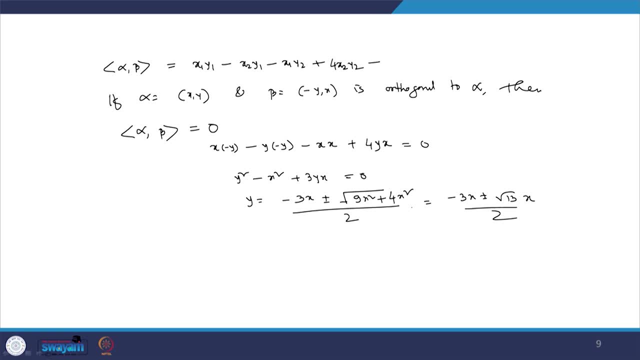 So y will definitely related by x in this way, please, Again, the space of say continuous function, another, let me take another examples. Let V be the space of all real valued continuous function in closed interval. say minus pi to plus pi, Then sin T is orthogonal to cos T. So this you can check it as a homework, please. 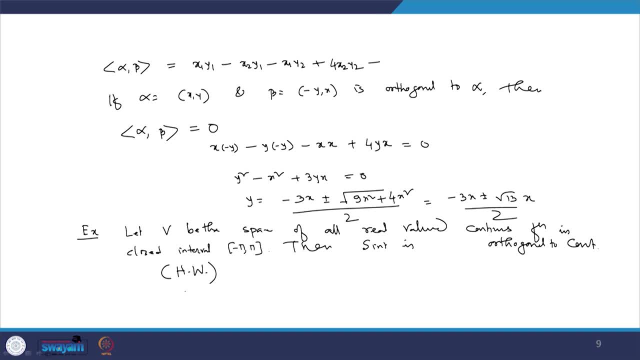 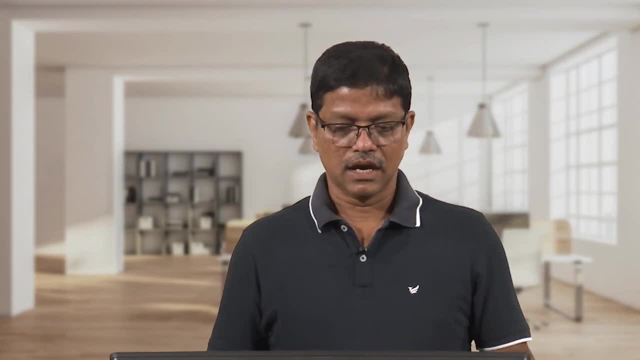 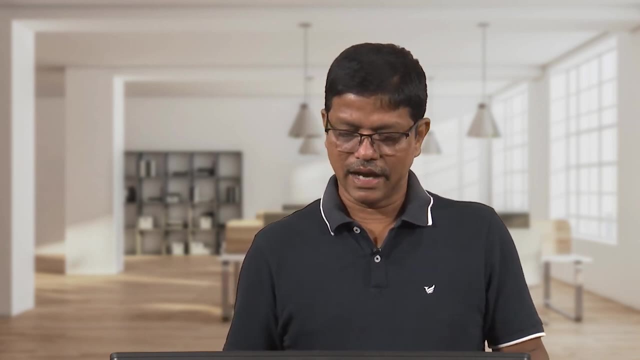 So we will discuss more about this- orthogonal sets and orthogonal vectors in our next class, please. So we see that the two vectors they will, if they are orthogonal, They have to satisfy such criteria. and then again we have seen that, you know, over the 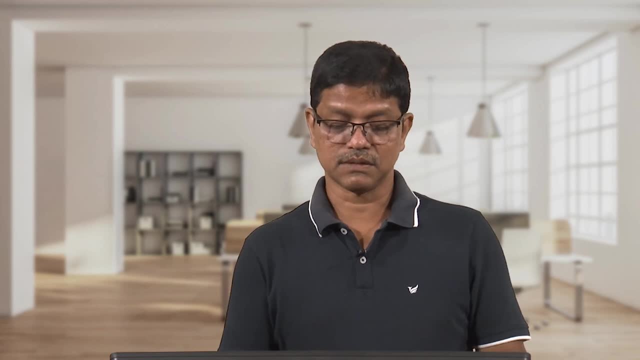 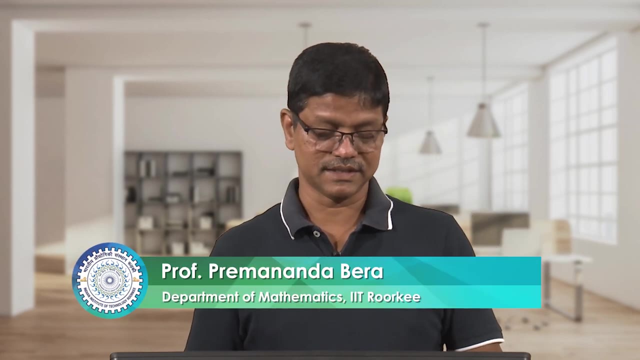 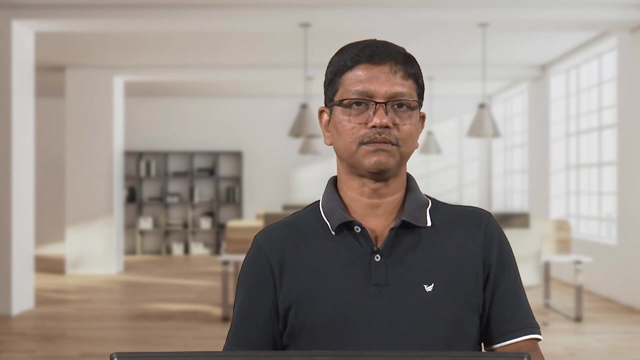 space of real continuous function in closed interval minus pi and plus pi. The function sin T is orthogonal to cos T or cos T is orthogonal to sin T, please. So we will discuss more on this. orthogonal sets in and some properties of this in our